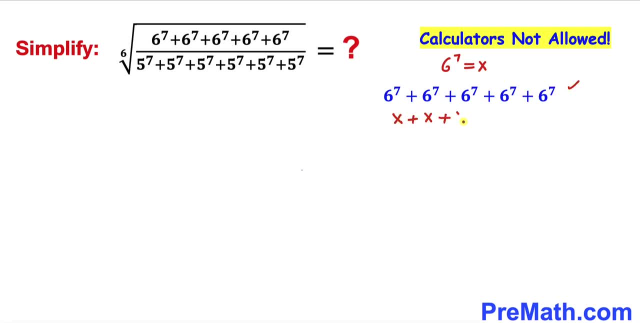 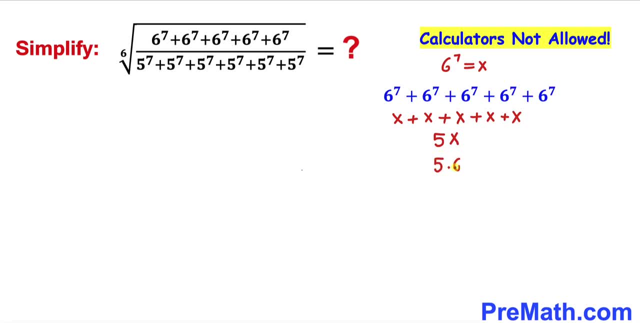 going to become 5 times 6 power 7.. So, therefore, this expression is same as 5 times 6 power 7.. Likewise, let's focus on this denominator part, and here I have copied it down, and now let's assume that this 5 power 7 is y. 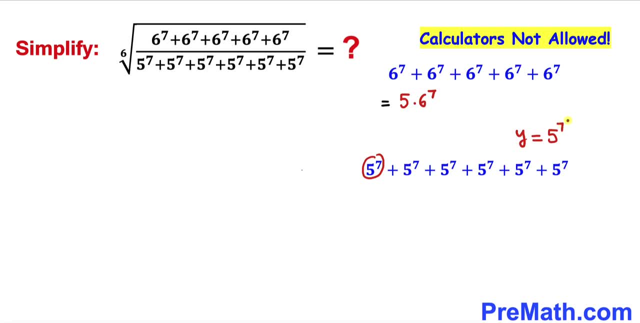 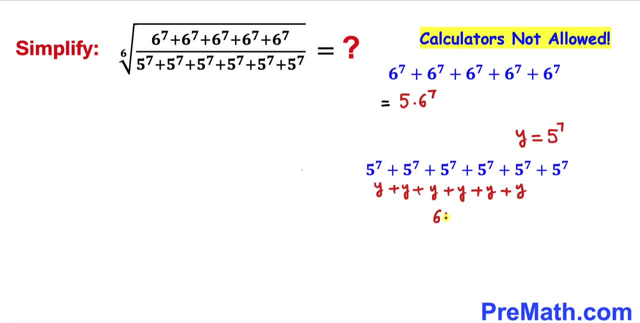 Let's combine all these y, So this is going to give us six times y. So we know our y is 5 power 7.. So therefore, I'm going to replace this y by 5 power 7.. So therefore, this could be written out 7 times 6 and we are going to give us 6 times y. 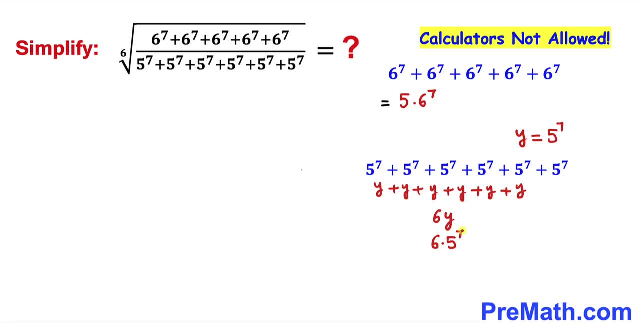 6 times 5 power 7.. So, therefore, this expression is equal to 6 times 5 power 7.. So, therefore, I'm going to replace this numerator by this 5 times 6 power 7, and this denominator by this 6 times. 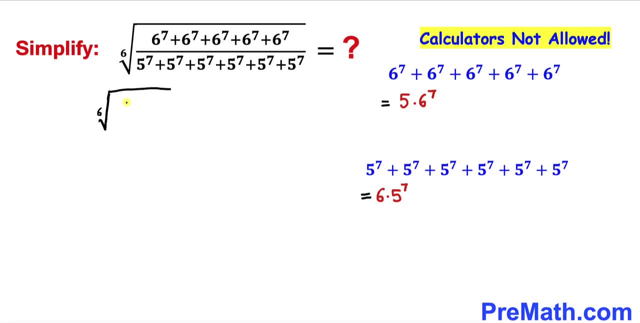 5 power 7.. So, therefore, we can write this sixth root of, and the numerator is going to be 5 times 6 power 7, divided by 6 times 5 power 7.. Now let me go ahead and put these: 5 and 5 power 7. 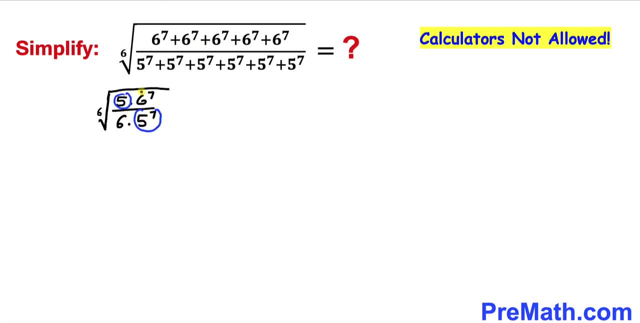 together, and likewise 6 power 7 and 6 together. So therefore this could be written as: 5 divided by 5 power 7 times 6 power 7 divided by 6.. And now we know that 5 is same as 5 power 1 and 6 is same as 6 power 1.. And now let's recall. 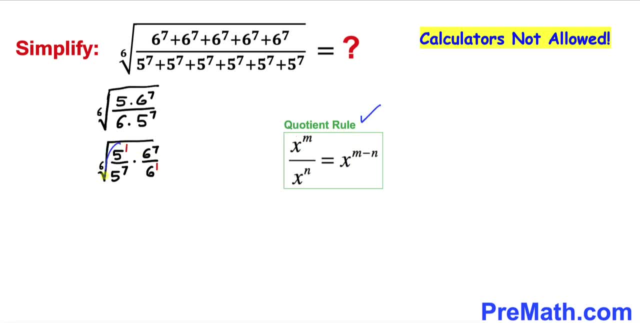 this quotient rule of exponents We are going to apply on these both parts. So, therefore, this is going to give us 6 power 7 minus 1 is going to give us 6 power 6. divided by likewise, this is going to give us 5 power 6.. And now we can break this one down. This could be written: 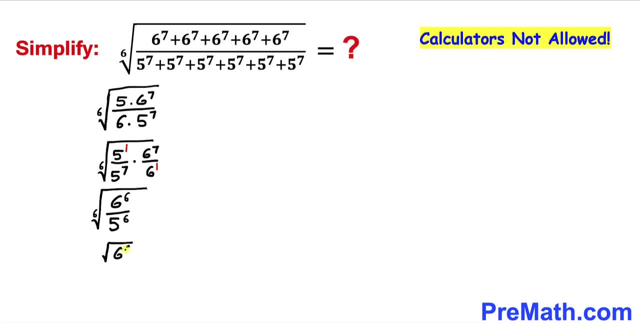 as 6 power 7 minus 1.. So, therefore, this is going to give us 6 power 7 minus 1, divided by 6 root of 6- power 6 divided by 6 root of 5- power 6.. And now let's recall this basic rule. 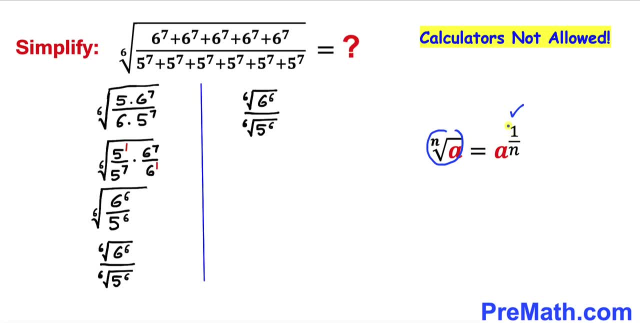 Nth root of a could be written as a power 1 over n. So therefore 6th root of a could be written as a power 1 over 6.. We are going to apply this property over here. So therefore our this numerator could be written as 6 power 6, and then whole power 1 over 6 divided by likewise. 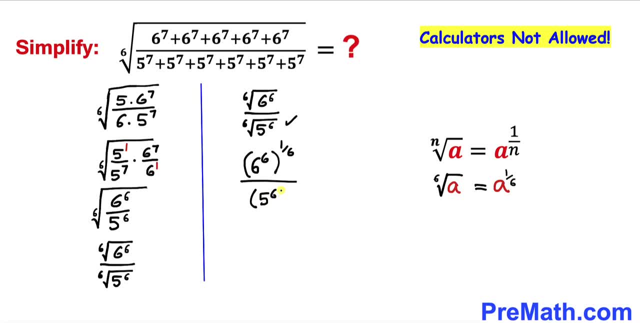 this could be written as 5 power 6 and whole power, 1 over 6.. Now let's recall the power rule of exponents. Whenever we have these nested exponents m and n, we can multiply them out. So therefore, if we multiply these nested exponents 6 times, 1 over 6 is going to give us 1.. 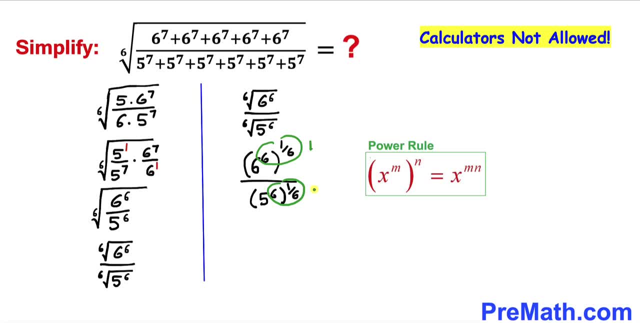 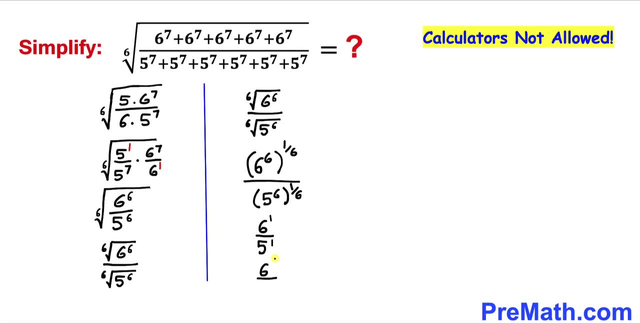 Likewise, 6 times 1 over 6 is going to give us 1 as well, As you can see in this next step. And now, 6 power 1 is same as 6. divided by 5 power 1 is same as 5.. And that's our simplified answer. 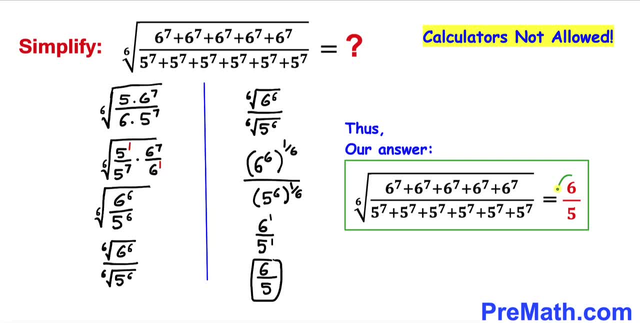 So thus our simplified answer to this given radical problem turns out to be 6 divided by 5.. Thanks for watching and please don't forget to subscribe to my channel for more exciting videos. Bye, Thanks for watching and please don't forget to subscribe to my channel for more exciting videos.